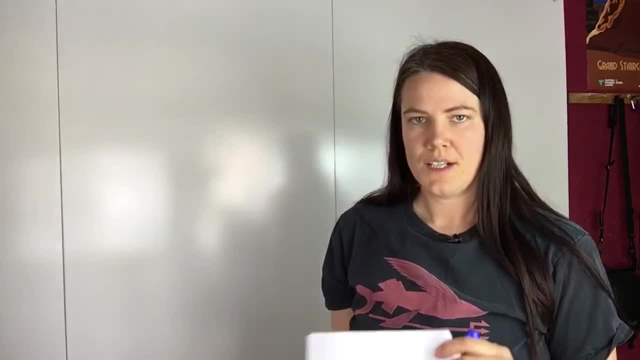 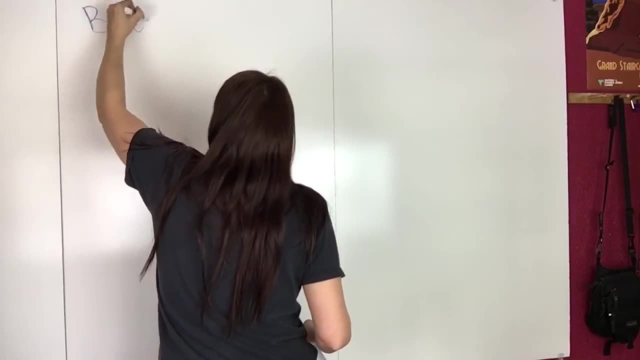 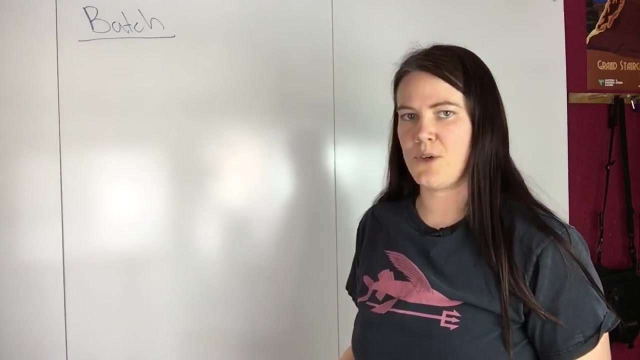 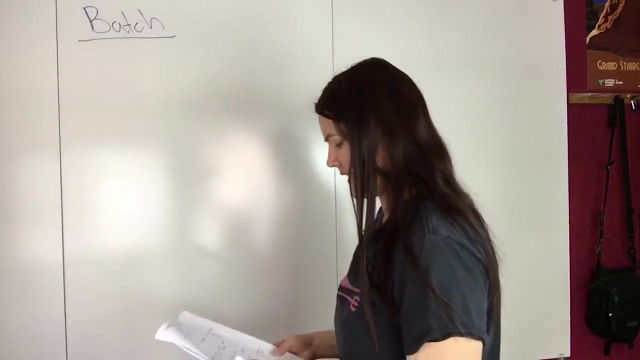 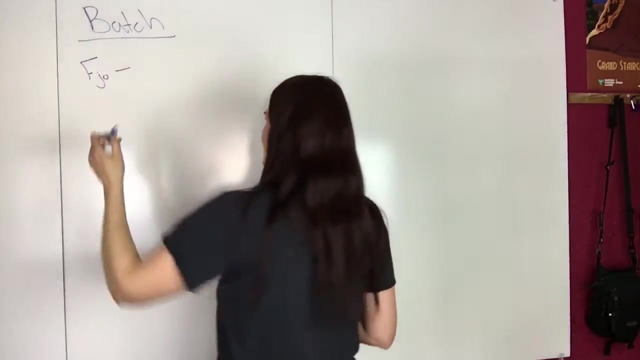 Alright. so in this video I wanted to talk about the mole balance for a batch reactor, So batch- And in the previous video I derived the general mole balance for reactor design. So I'll just write that down real quick. So we had Fj- naught whatever's flowing in, minus Fj- whatever's flowing out. 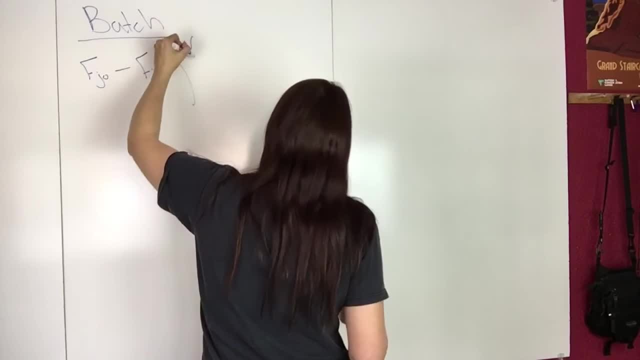 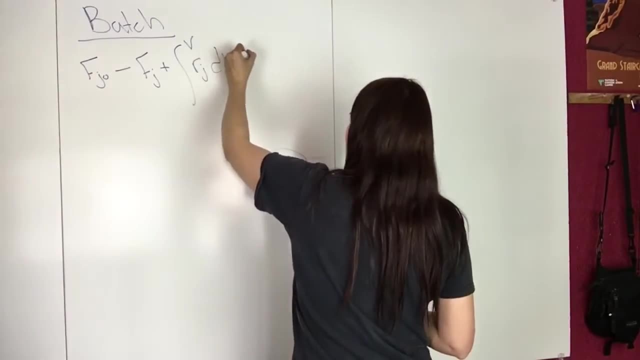 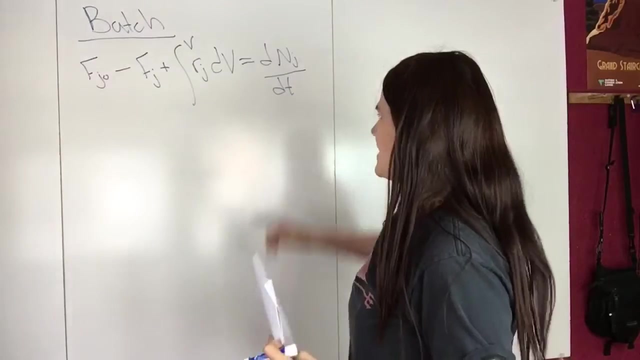 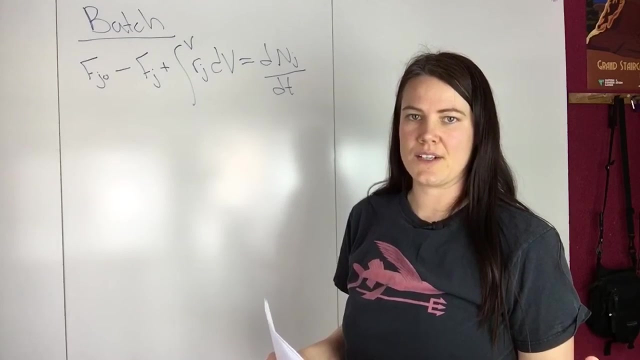 plus the integral of V, Rj, dB. whatever's being generated inside the reactor equals dNj, dt, So whatever's accumulating. So if you think about a batch reactor, you know that there's nothing flowing in or out. 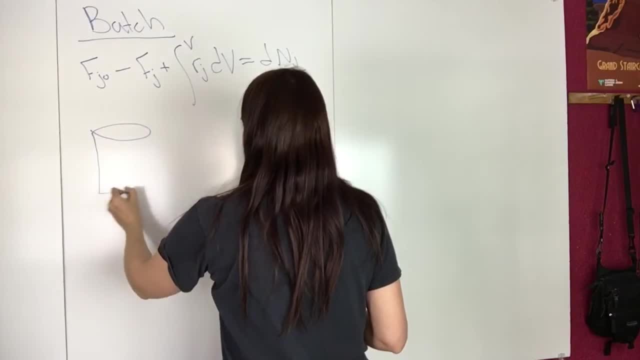 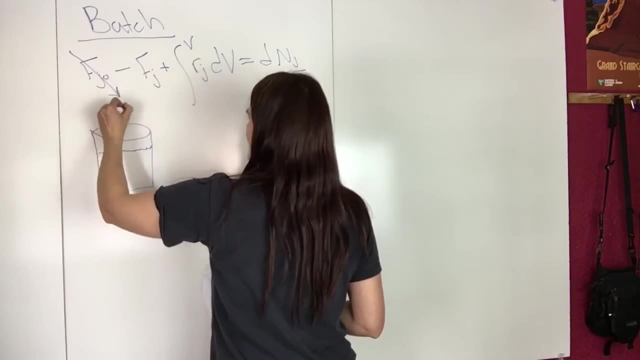 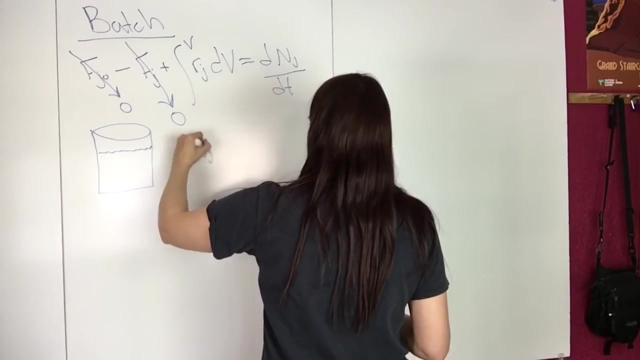 You just have this, So right away you can see that this term is zero and this term is zero. So you're left with dNj, dt. equals dNj, dt, equals, dNj, dt, equals Rj. 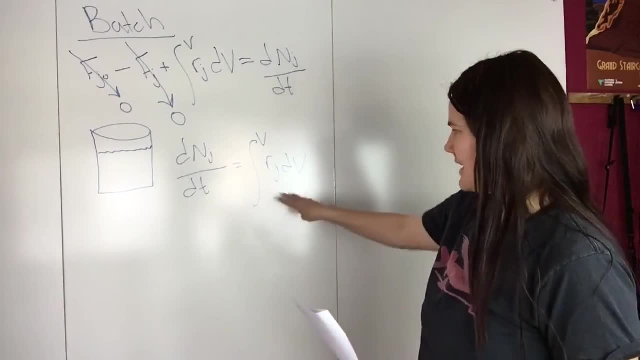 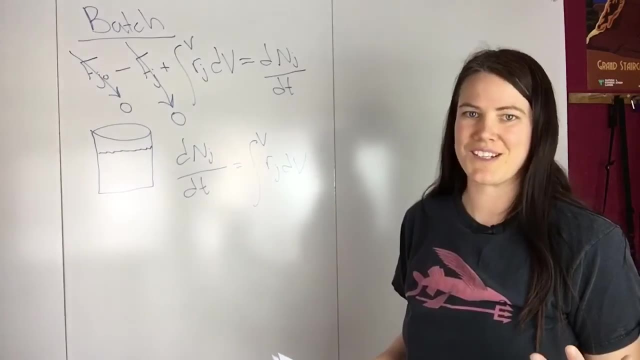 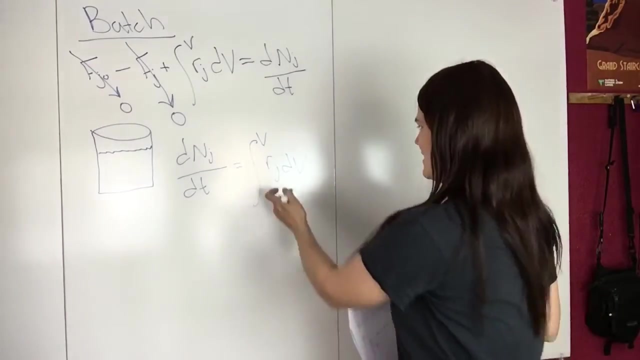 dV. And then, looking at this, if you know, you can make another assumption- If you know that this is perfectly mixed- so basically the rate isn't a function of position because everything's perfectly mixed- then you can pull this out of the integral. 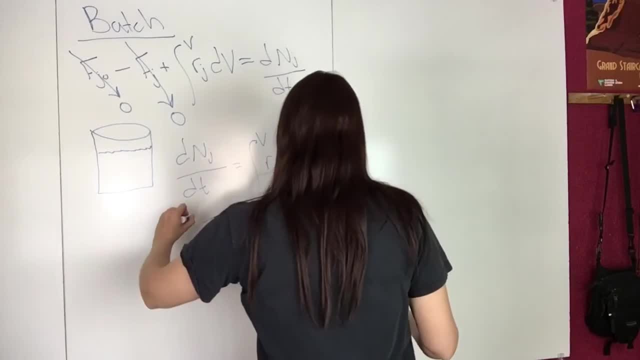 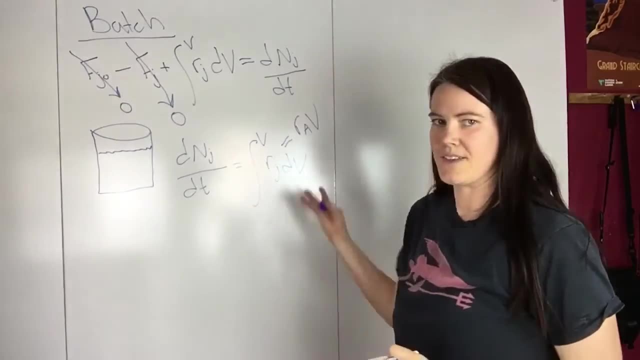 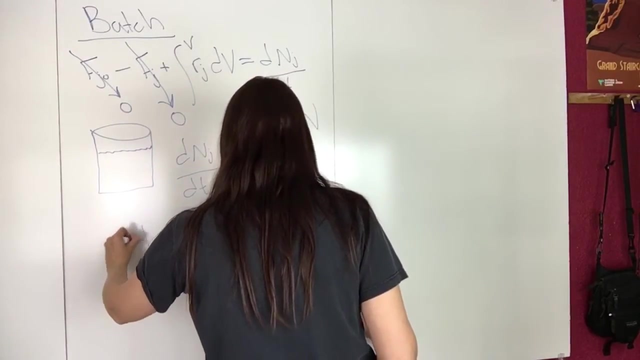 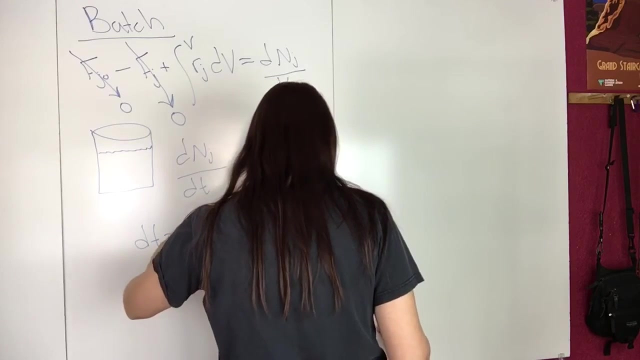 so then you end up with: well, this can turn into this, Because you pull Rj out, and then this is what you're left with, And so then you? so then you can rewrite this as dt equals dNa. Well, okay, and I also kind of switched the j to an a. 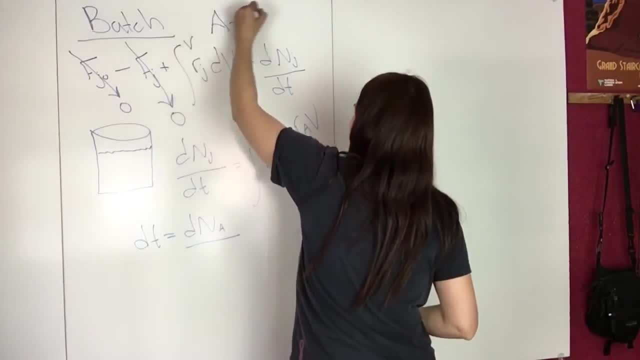 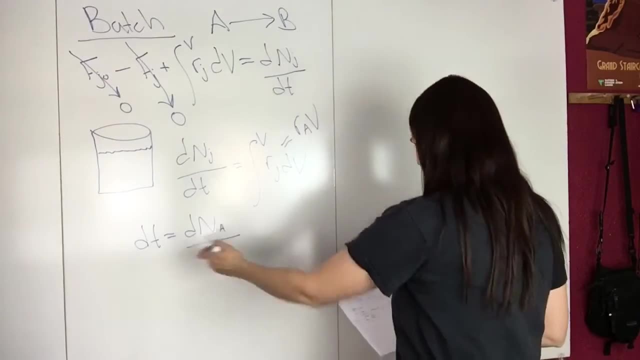 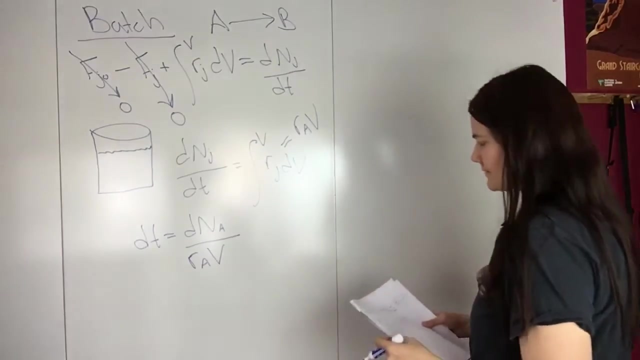 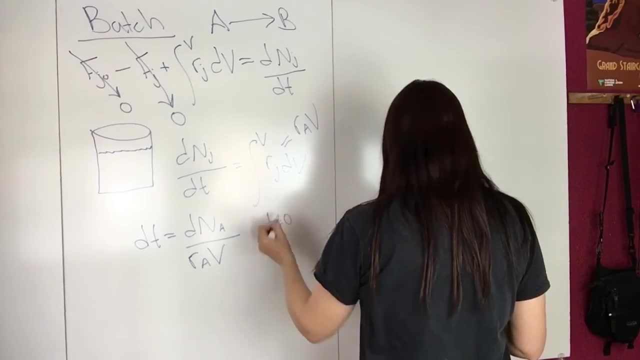 So, assuming that you have a reaction that looks like this, let's just assume that we're looking at a So dt dNa Ra over V, And then we can integrate with the following limits: We want to integrate from: t equals zero.